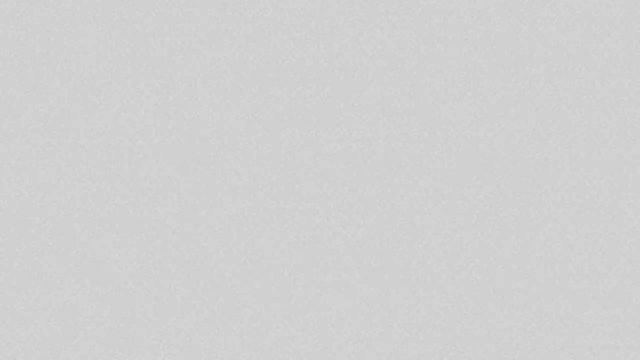 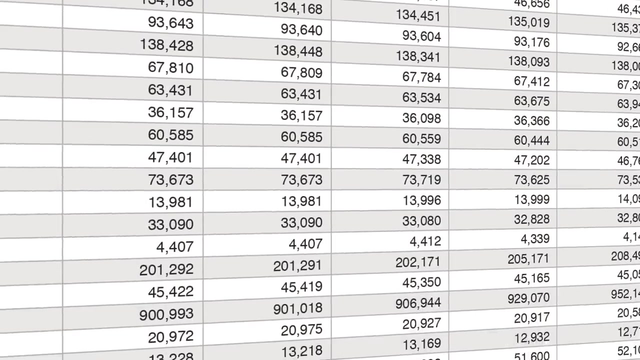 such as age and gender distribution. So how can we keep track of all that data in a way that makes it easy to comprehend? Complex data is more easily interpreted through visualization and one of the ways that demographers represent the internal distribution of a population. 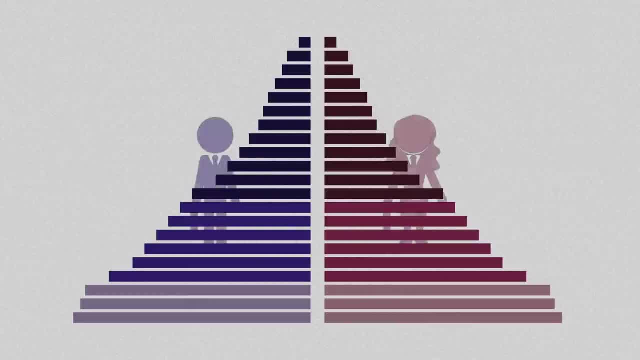 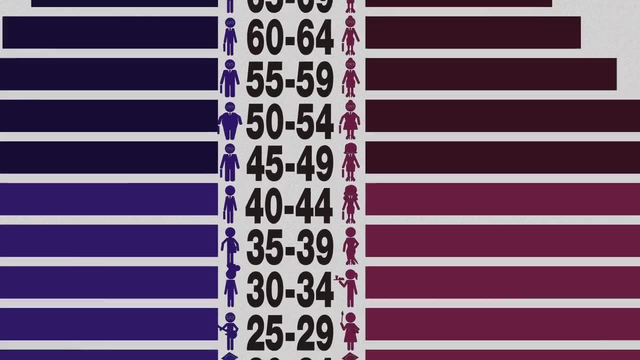 is the population pyramid. Here the data is divided by gender, with females on one side and males on the other. The population numbers are shown for each five-year age interval, starting from zero to four and continuing up to 100 and up. 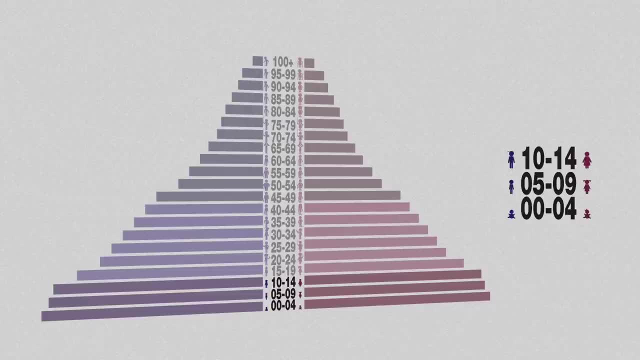 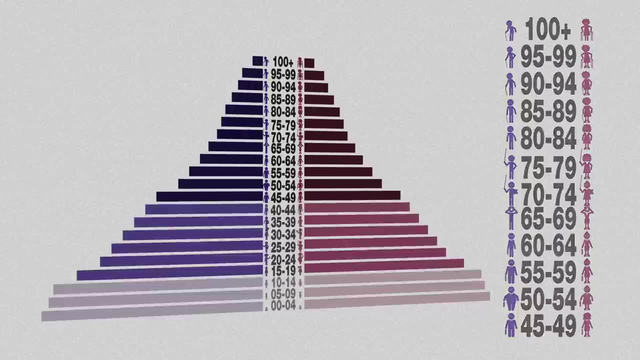 These intervals are grouped together into pre-reproductive zero to 14, reproductive 15 to 44, and post-reproductive years 45 and up. Such a population pyramid can be a powerful predictor of future population trends, For example. 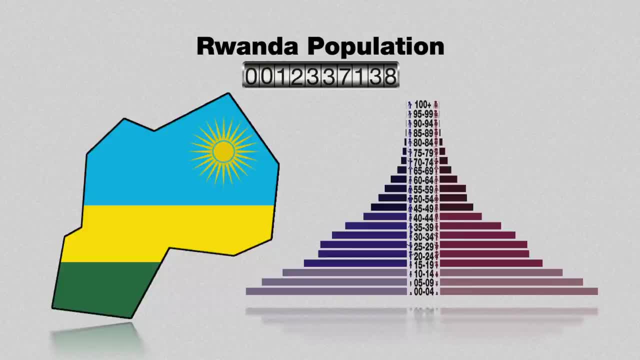 Rwanda's population pyramid shows it to be a fast-growing country, With most of the population being in the youngest age groups, at the bottom of the pyramid. the number will grow rapidly in the coming years As today's children reach their reproductive years and have children of their own. 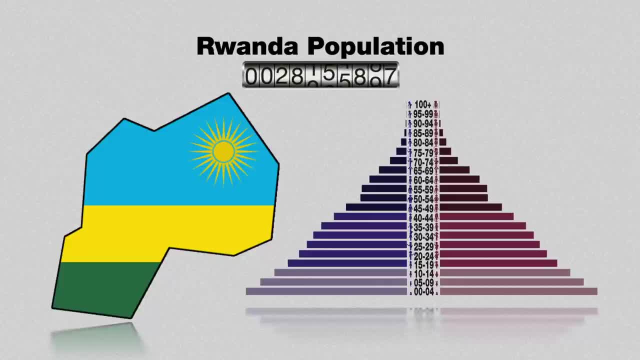 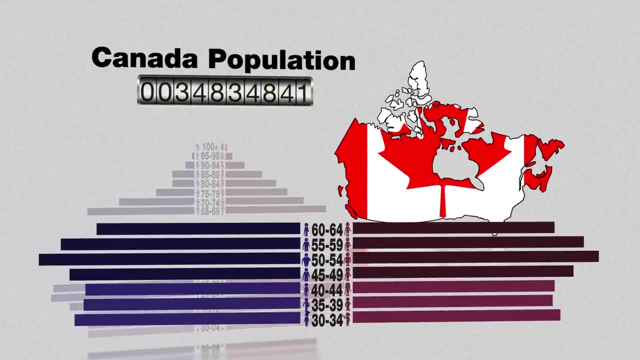 the total population is almost certain to double within the next few decades. For our second example, let's look at Canada, where most of the population is clustered around the middle of the graph, Because there are less people in the pre-reproductive age groups. 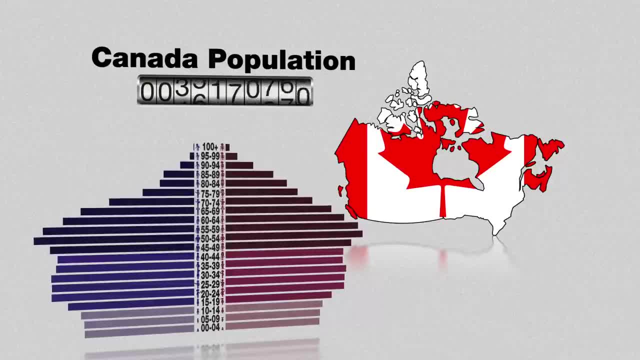 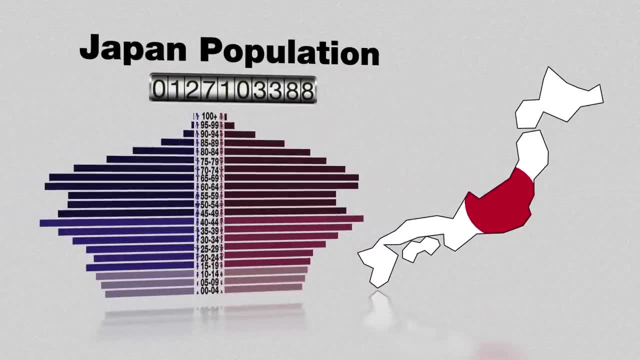 than there are in the middle of the graph, Because there are less people in the pre-reproductive age groups than there are in the reproductive ones. the population will grow more slowly as the number of people reaching their reproductive years decreases. Finally, let's look at Japan. 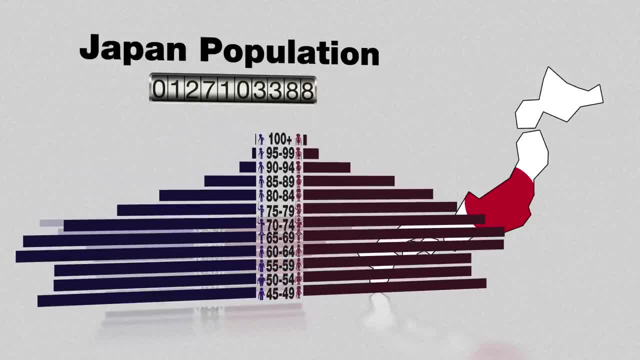 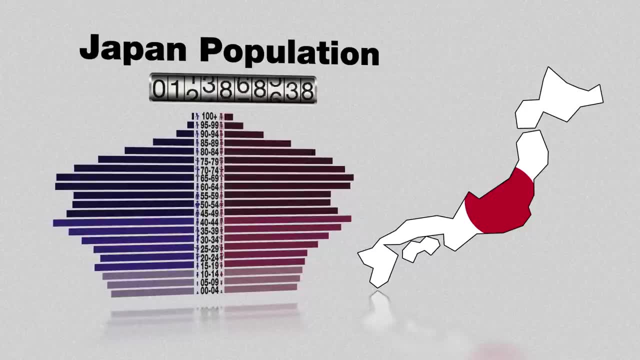 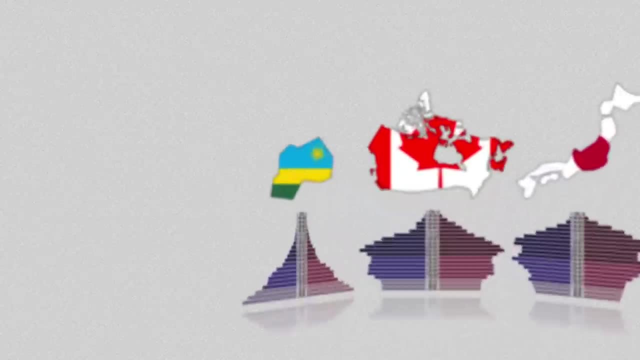 Because the majority of its population is in its post-reproductive years and the number of people is smaller at each younger interval. this means that at current rates of reproduction, the population will begin to decline as fewer and fewer people reach reproductive age. Comparing these three population pyramids side by side: 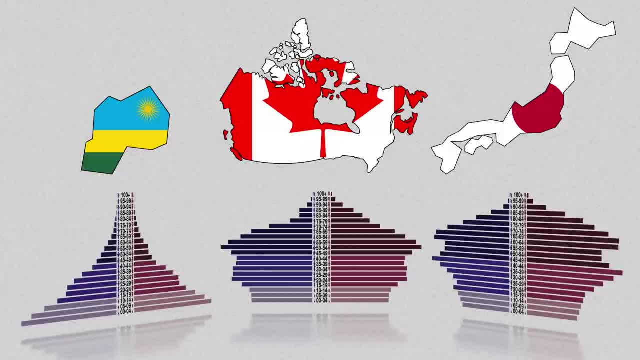 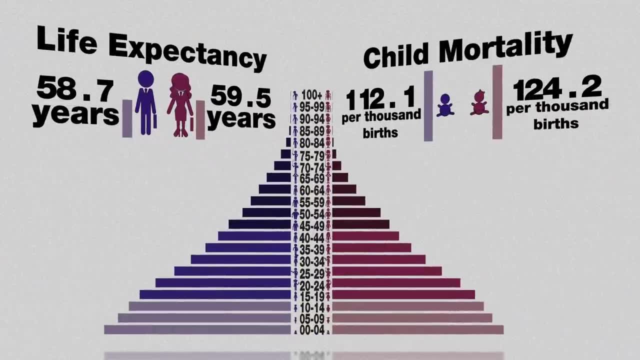 shows us three different stages of demographic transition as a country moves from a pre-industrial society to one with an industrial or post-industrial economy. Countries that have only recently begun the process of industrialization typically see an increase in life expectancy and a fall in child mortality rates.